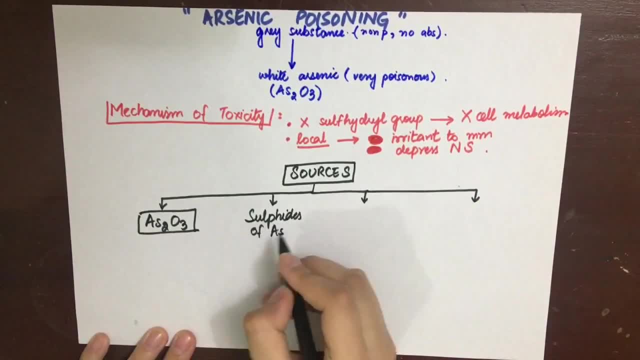 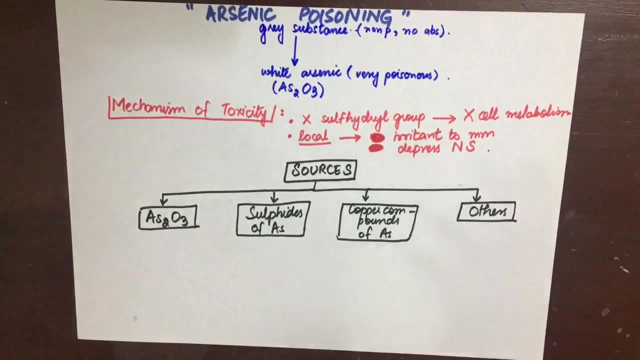 is arsenic trioxide. next will be sulfides, then will be copper, compounds of arsenic and some others, now the arsenic trioxide. it basically occurs in two forms. one is the crystalline white powder form and the second is opaque, brittle mass. like it resembles enamel. they're also called Sankhya or Somalkar. 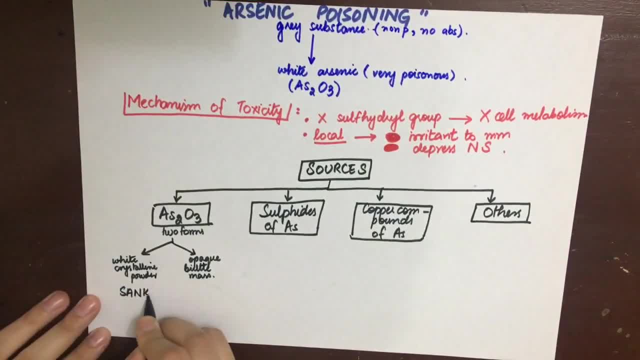 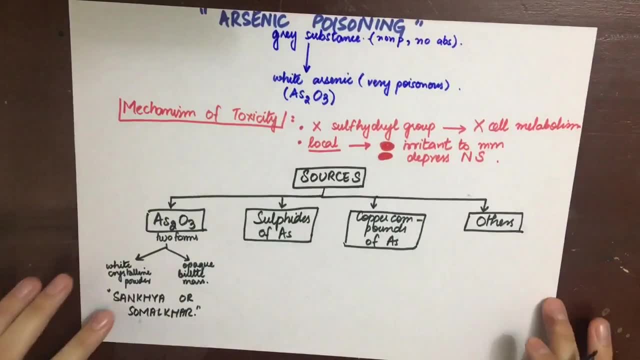 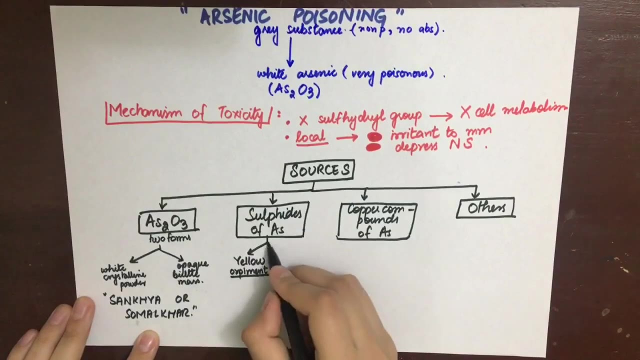 locus. they have no smell or taste, are sparingly soluble in water and float when mixed with milk, coffee or tea. the sulfides of arsenic mainly occur in two forms: a yellow or pigment, which is basically a yellow to orange sulfide of arsenic, and a red real girl, which is a red sulfide of arsenic. 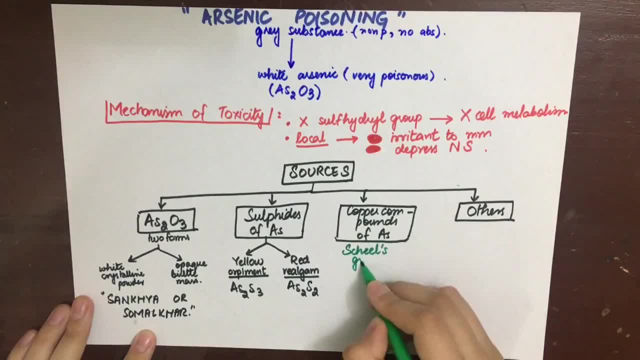 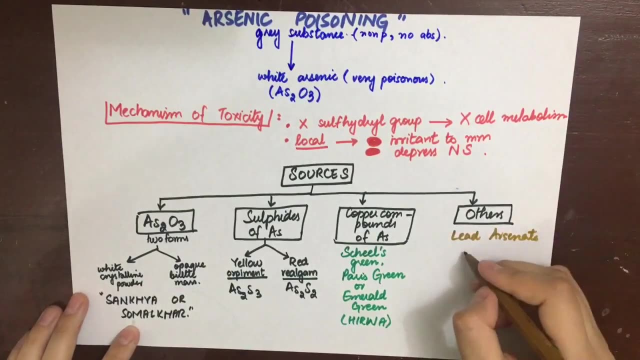 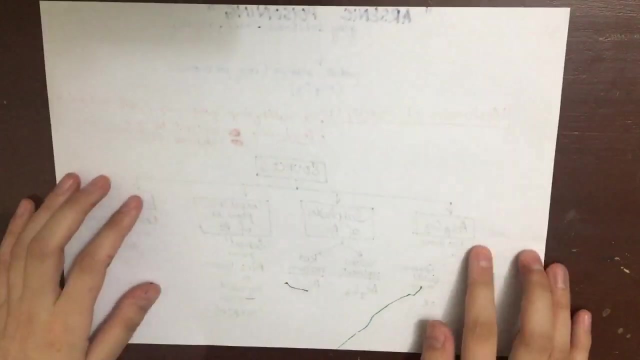 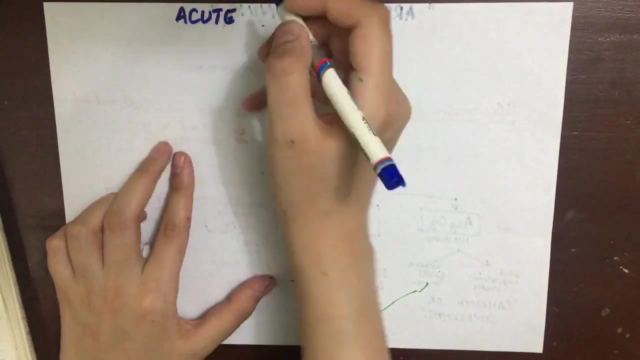 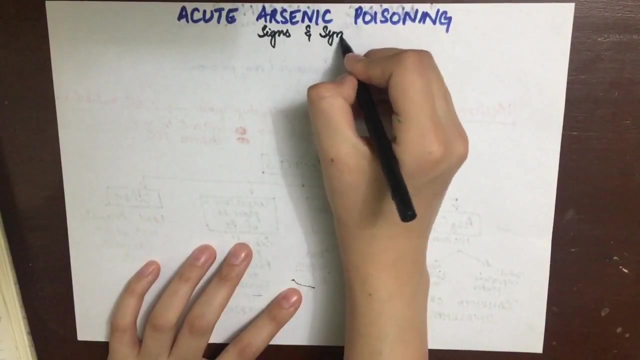 the copper compounds are mainly shields green, Paris green or emerald green and are known locally as hero. others include lead arsenate, sodium arsenate and potassium arsenate, etc. let's now discuss acute arsenic poisoning and then we'll discuss chronic arsenic poisoning. sign in symptoms of acute arsenic poisoning can be divided into three time. 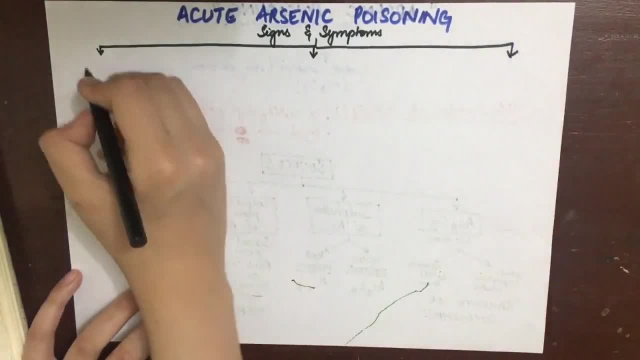 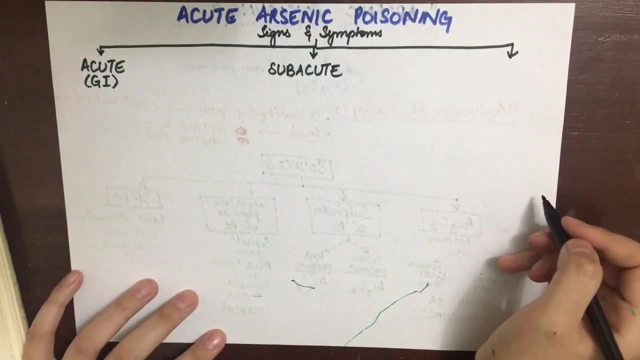 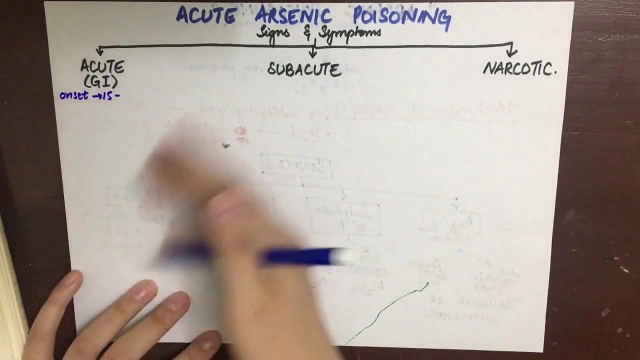 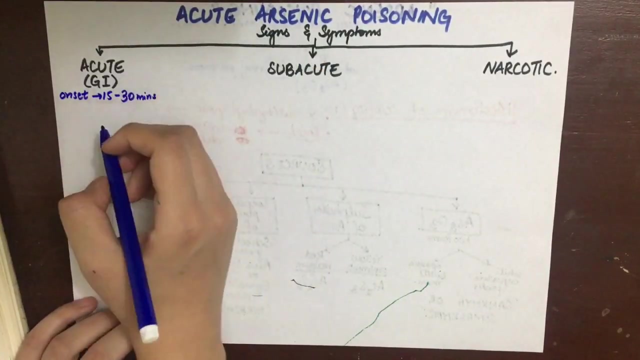 zones or depending on the onset of symptoms and whether they have remission or not. one is a cute which is mainly on the GI, second is a acute and then is narcotic. the onset of the acute GI syndrome symptoms start in about 15 to 30 minutes of ingestion and if there is food in. stomach. the symptoms may be delayed and death occurs in one to two days. the sub acute symptoms will cause seven to ten days, and the narcotic form will cause death in two to three hours. now, the acute GI symptoms are the same as that of an irritant poison, that is, burning pain in stomach, esophagus and 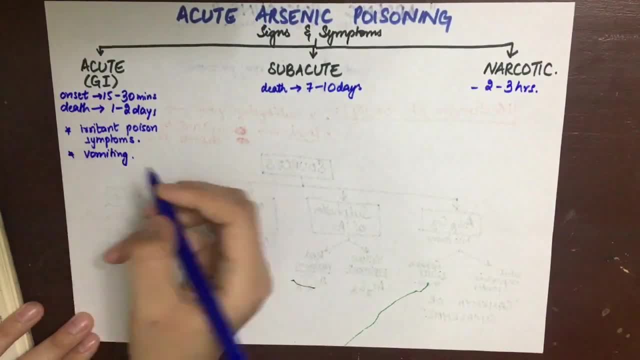 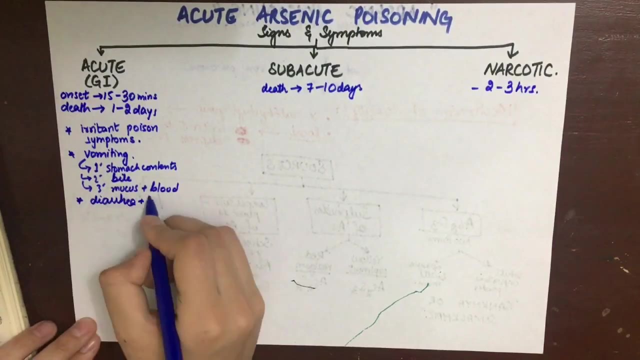 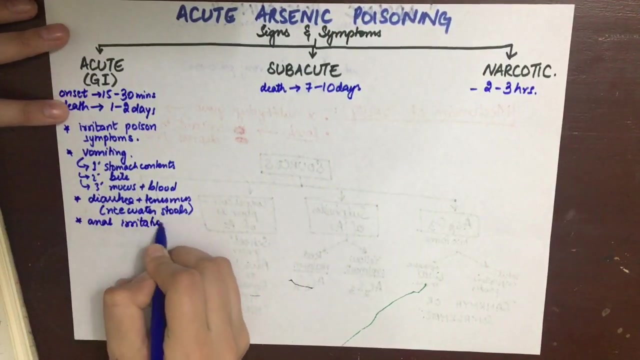 epigastrium and severe, continuous vomiting. at first the warmatic contains the stomach contents, food, etc. later there is bile and finally they can be mucus and blood in the warm attis. the diarrhea is accompanied with tenesimus and the diary resemble rice water stools. is also blood tinged with shreds of. 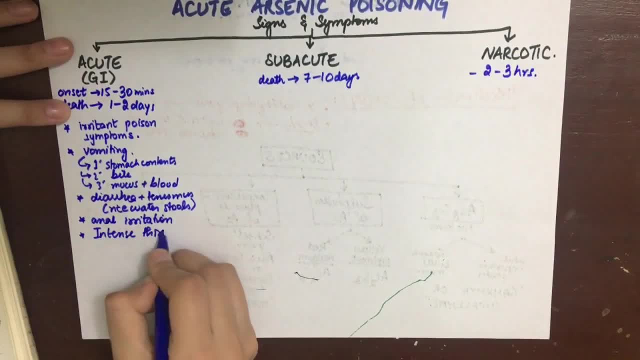 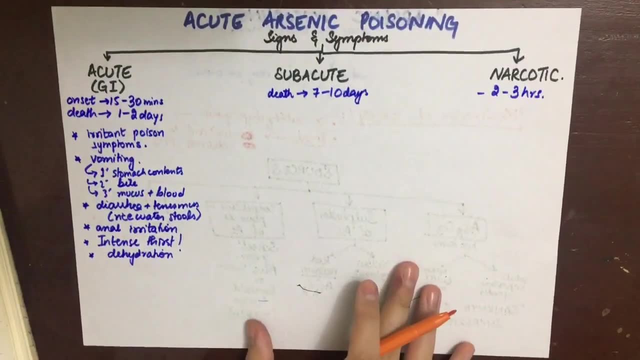 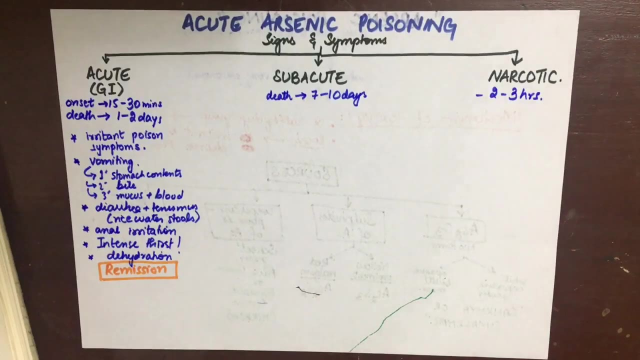 poison fragments and mucous membranes. there is année Irritation, increased thirst and when you drink water it causes more vomiting. Painful cramps are there due to dehydration. There can be a period of remission when the patient feels okay, and then the patient can collapse. 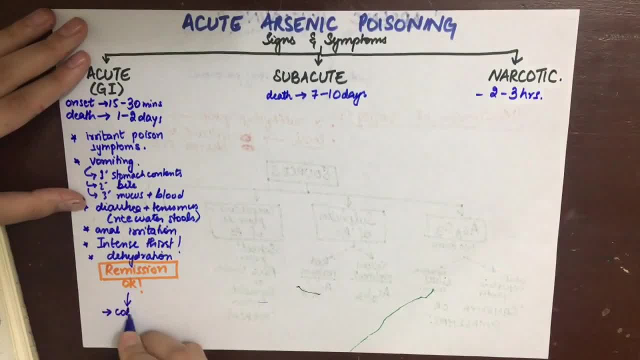 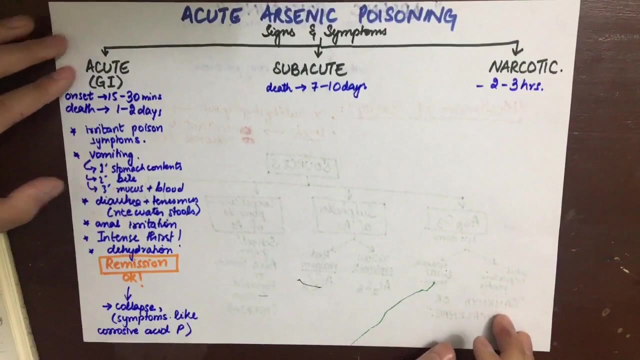 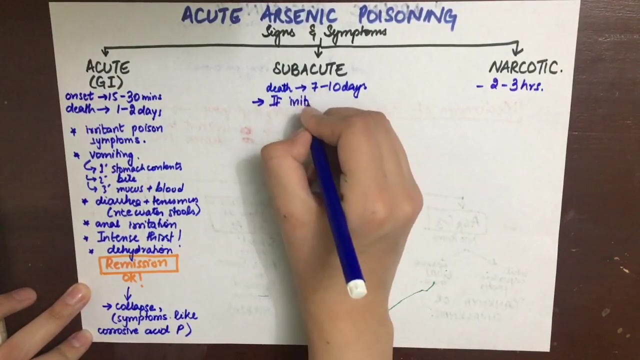 Having the same symptoms like those we discussed in corrosive acid poisoning, that is, pale, anxious face, sunken eyes, dilated pupil, rapid, feeble pulse, increased respiratory rate and convulsions in death. Now the subacute poisoning occurs if the patient survives the acute attack. 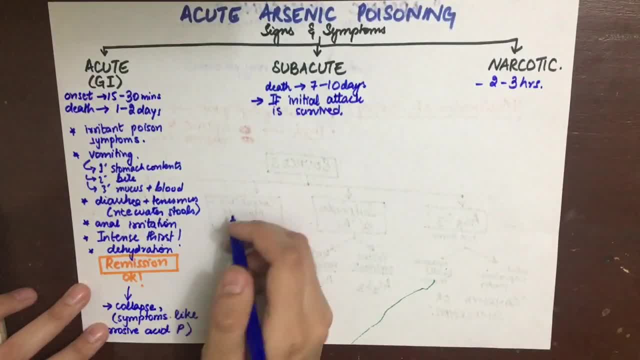 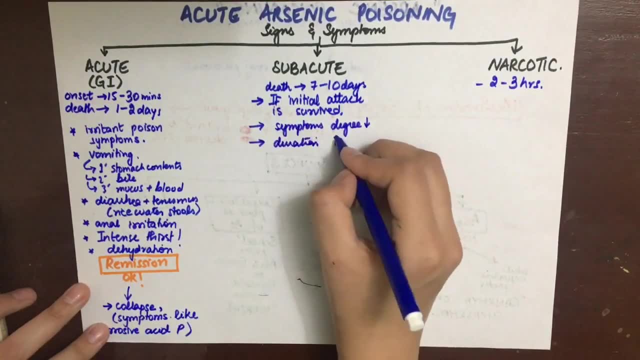 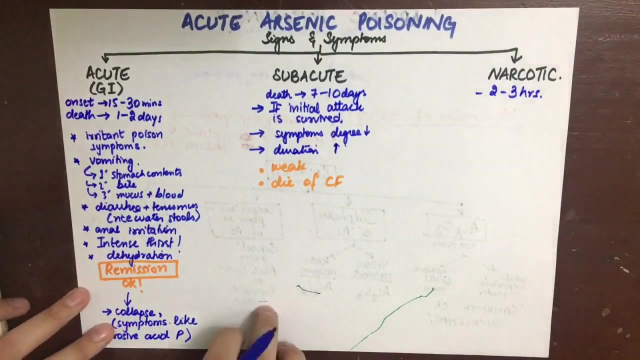 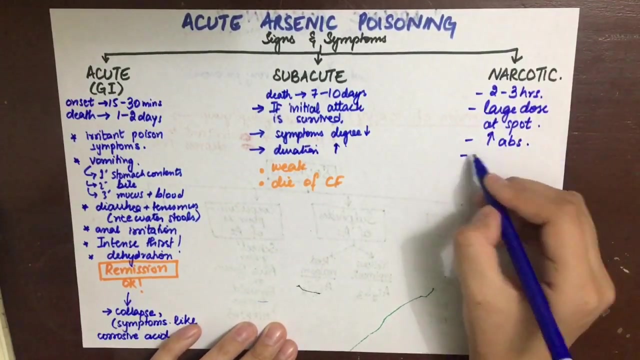 The degree of the symptoms is decreased, that is, the symptoms are less severe, but the duration is increased. The patient is weak and at last die of cardiac failure. Now the narcotic type of acute poisoning is when a large dose of arsenic is ingested. 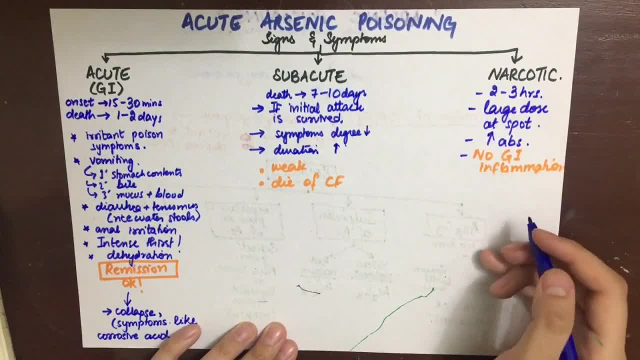 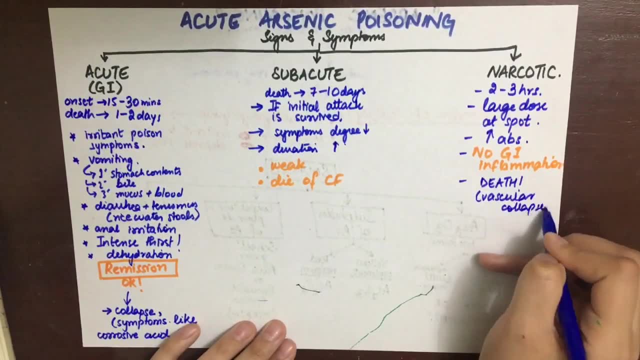 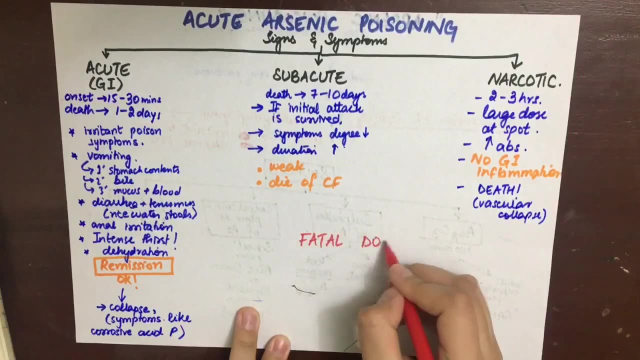 such that, before there can be absorption and gastric inflammation due to irritation, The patient dies of symptoms like vertigo, headaches, spasms, stupor and vascular collapse. Now the fatal dose and fatal period. The fatal dose is 120 to 200 milligrams in the adult. 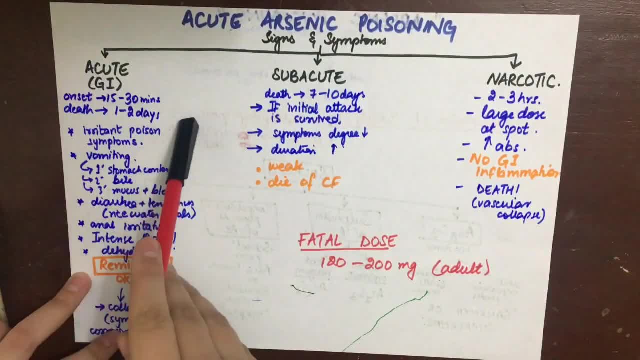 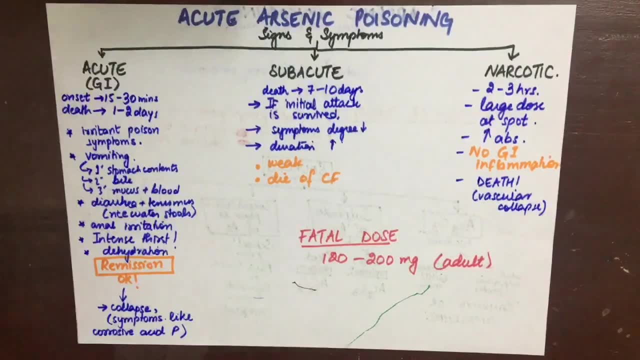 The fatal period is about 15 to 20 minutes in acute GI, 7 to 10 days in subacute poisoning, and narcotic poisoning in 2 to 3 hours causes death. Now the treatment for acute arsenic poisoning includes stomach wash with milk or warm water. 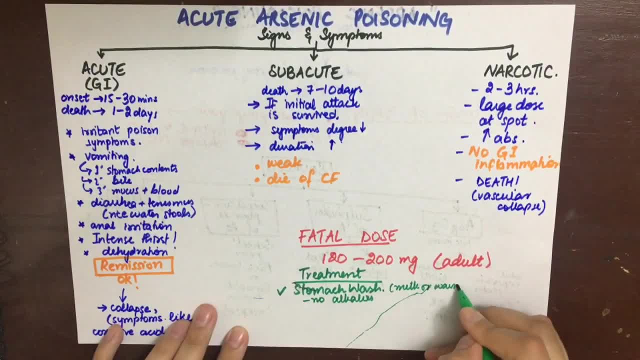 Alkalis should not be given because they increase the absorption by increasing the solubility of white arsenic. Freshly precipitated ferric oxide is the antidote for arsenic poisoning because it converts the arsenic into ferric arsenate, which is harmless. 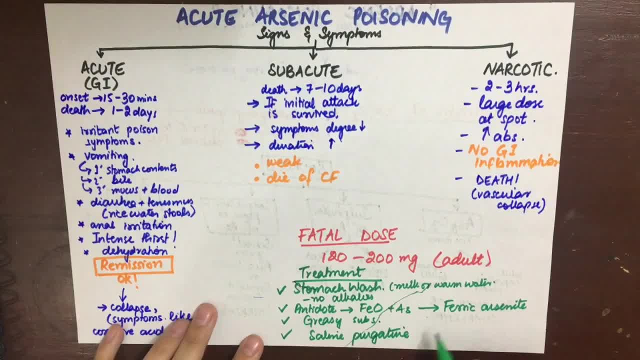 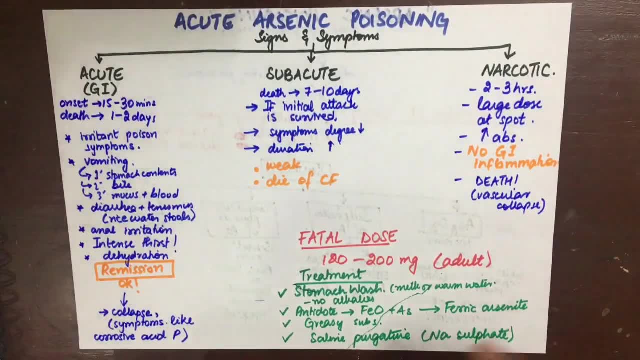 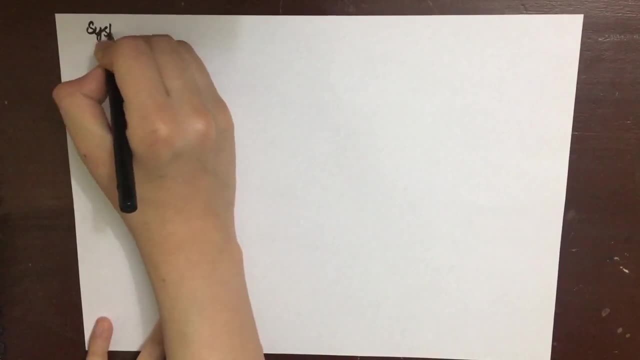 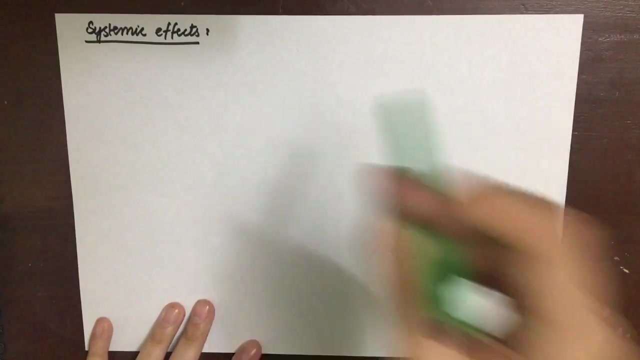 If it is not present, charcoal or calcined magnesia can be given Butter and grease to prevent absorption, and saline purgatives such as sodium sulfate. Now the systemic effects are combated by giving IV, British antileucite agent. 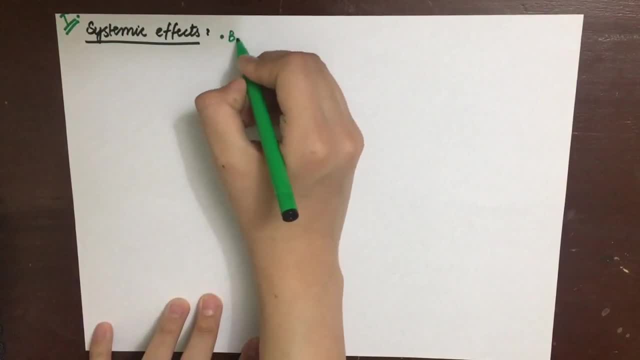 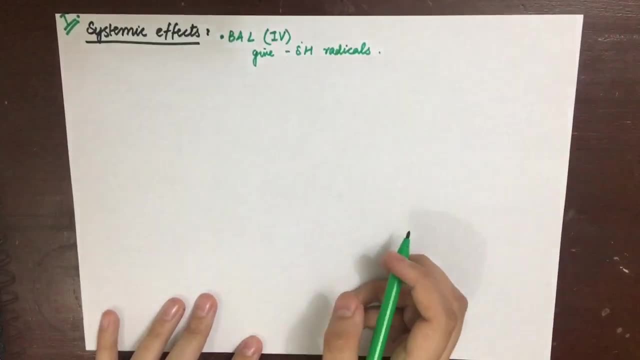 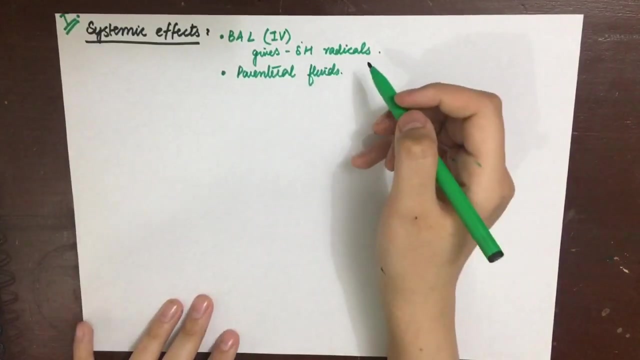 Now, the mechanism by which BAL acts is that it provides two sulfhydryl group agents, The sulfhydryl group radicals, to combine with the free arsenic and dislodges the arsenic from sulfhydryl groups. of the enzymes, The BAL arsenic complex is excreted by the kidneys. 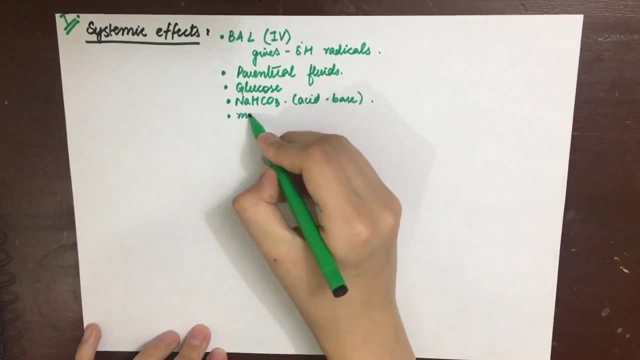 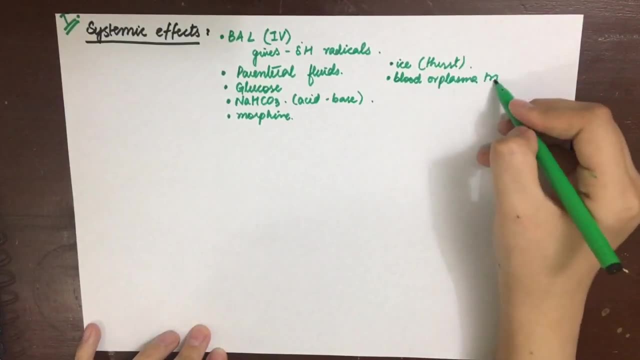 Parental fluids should be given for dehydration, glucose to protect the liver, sodium bicarbonate for acid-base balance, morphine for pain, ice to suck on for thirst relief, blood or plasma transfusion if necessary, And dialysis should be given to combat anuria. 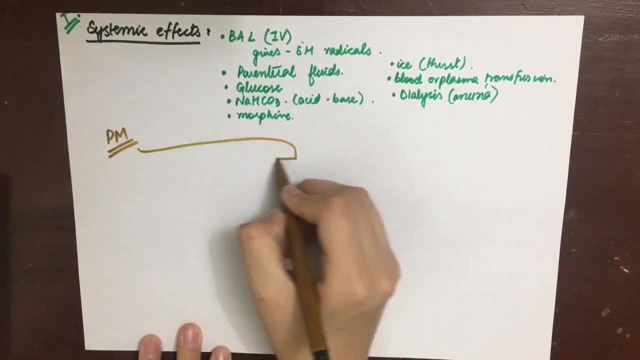 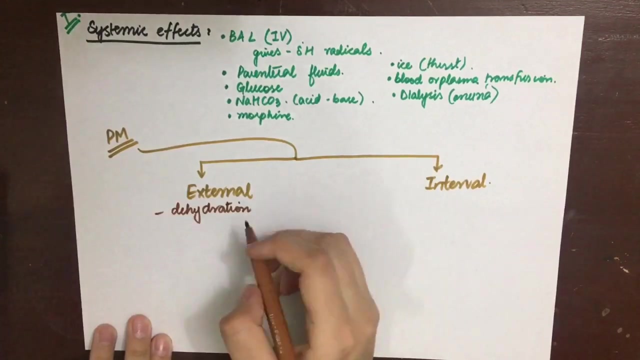 Now, the post-mortem findings of acute arsenic poisoning can be divided into external and internal findings. Externally, the dead body will appear dehydrated, with sunken eyes and wrinkled skin. The skin will be cyanosed and jaundiced due to liver compromise. 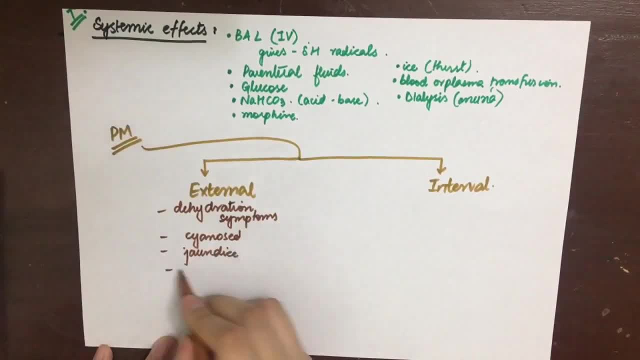 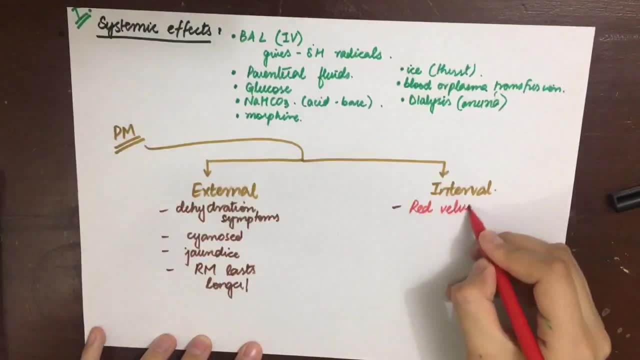 And rigor mortis will last longer in arsenic poisoning. Internal findings include characteristic red, velvety stomach. the mucosa appears red, edematous, swollen in patches. It has blood and mucus in it and submucosal petechial hemorrhages can be seen. 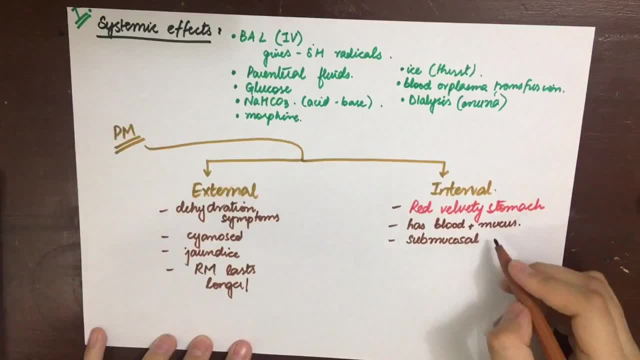 Rectum is most prone to inflammation. Sub-endocardial petechial hemorrhages can be seen. Hemorrhages in the larynx, trachea and lungs are also seen. Fatty degeneration of the liver is seen, which probably contributes to the jaundiced appearance of the dead body externally. 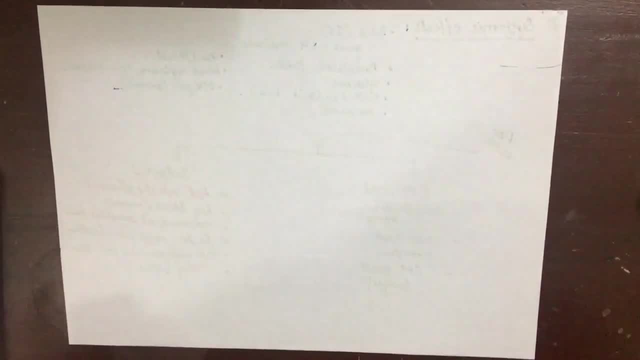 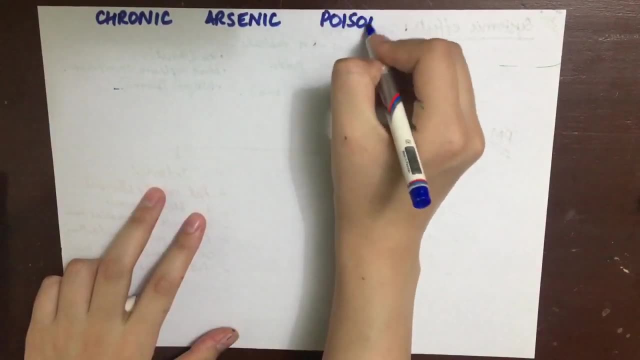 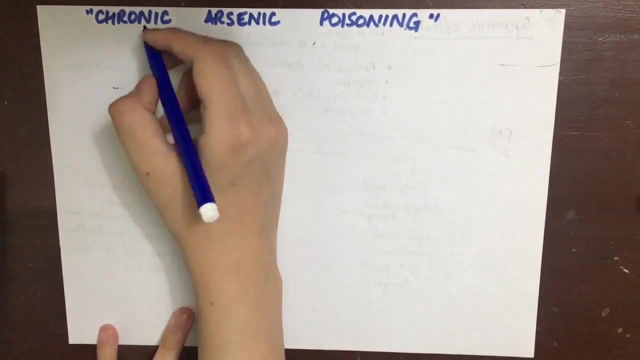 Now let's look at the chronic arsenic poisoning. Now, in what instances will chronic arsenic poisoning occur? Firstly, it can be an aftereffect of acute poisoning of arsenic. Secondly, it can be ingested in small doses over time. Thirdly, it can be taken in contaminated water or food. 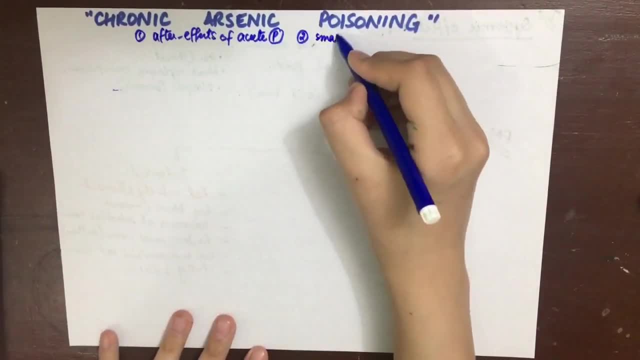 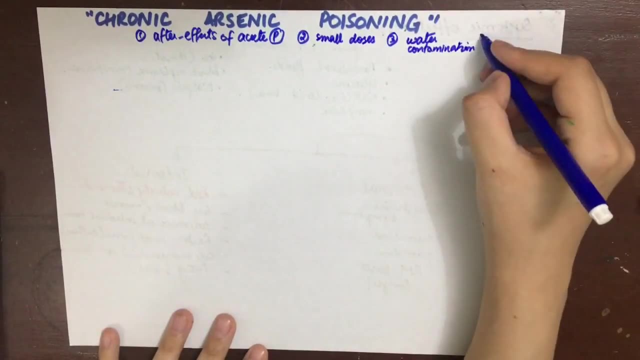 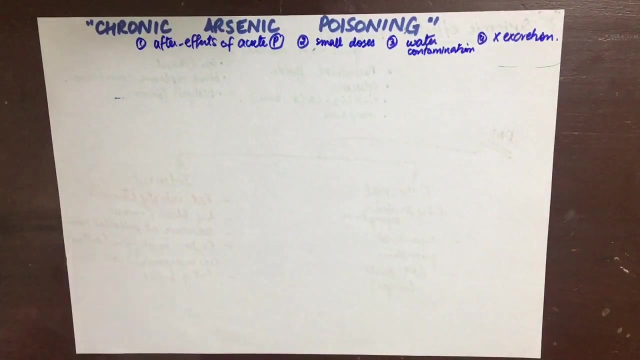 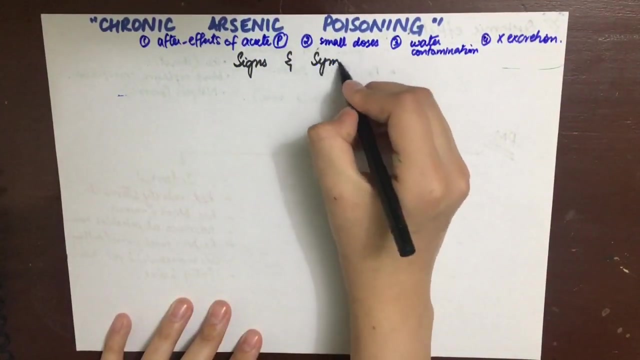 And fourthly, it can be due to compromised excretory capacity of the body. What are the causes of chronic arsenic poisoning? Now let's see how chronic arsenic poisoning manifests. The signs and symptoms of chronic arsenic poisoning can be divided into four stages. The first stage is of nutritional and GIT disturbances. The second stage is of catarrhal changes. Third is the skin rash stage And the fourth is nervous disturbances. Now the GI disturbances stage. the first stage is manifested as loss of appetite, nausea, vomiting and diarrhea. And these can be misdiagnosed, of course. The second stage of catarrhal changes resemble common cold-like symptoms. They might manifest as conjunctivitis, runny nose, coughing, etc. And bronchial catarrh can be seen which is simply fluid in the bronchus. 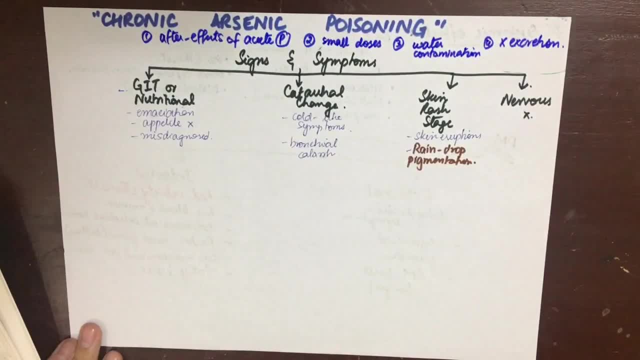 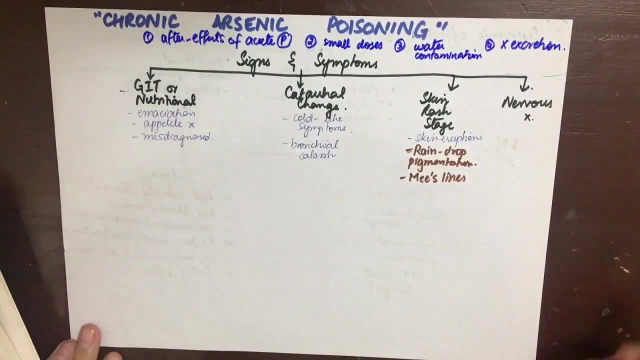 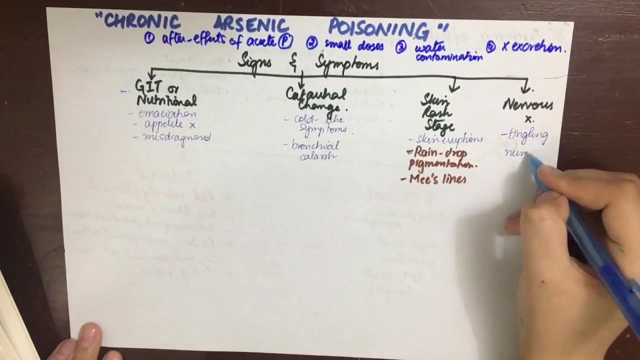 Skin rashes can manifest as raindrop pigmentation, which is a very characteristic finding in arsenic poisoning. Mies lines can be seen because there are periods of arrested growth due to interference with normal metabolism. Fourth stage mainly manifests as numbness, tingling and sometimes paresis. Arsenical neuritis closely resembles that associated with chronic alcoholism, and thus this can be misdiagnosed as well. Now, the treatment for chronic arsenic poisoning is that the exposure of the patient should be immediately disconnected. British antiluosite agent should be given. 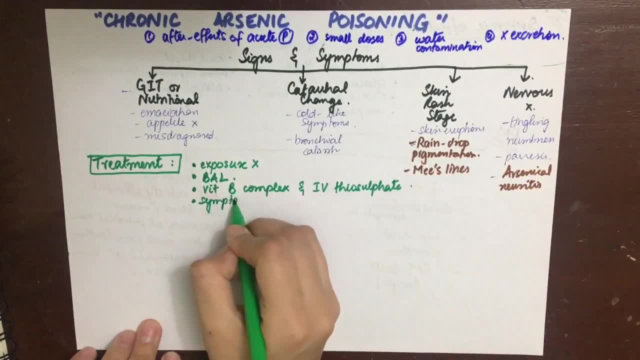 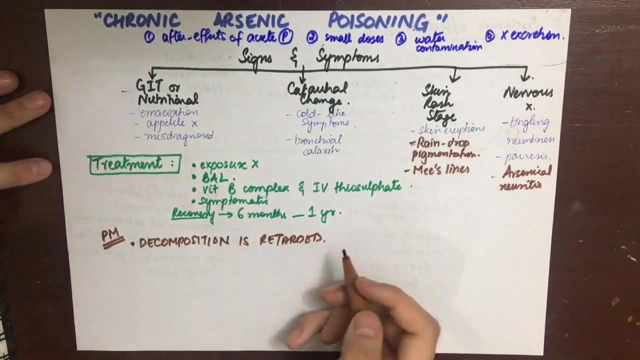 For the same reasons as mentioned before. Vitamin B complex and IV thiosulfate is given, Symptomatic treatment is given and recovery is about in six months to one year. Now the post-mortem changes is that. one change that you should remember is the decomposition of the body is retarded. The body looks emaciated, Anemic, fatty changes are seen in the liver muscle, heart and liver Skeletal muscle. There is congestion of the GIT. Why? Because liver is cirrhosed, So portal blood pressure is increasing and leads to congestion of blood in the GIT. 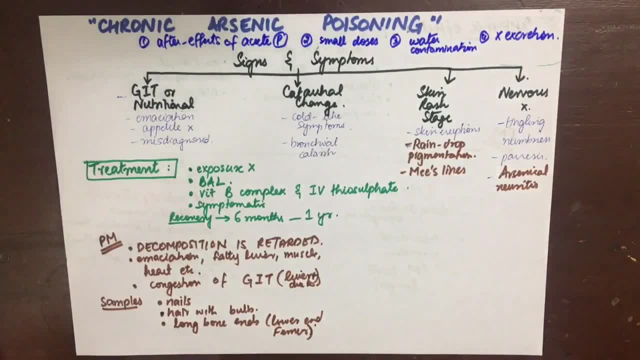 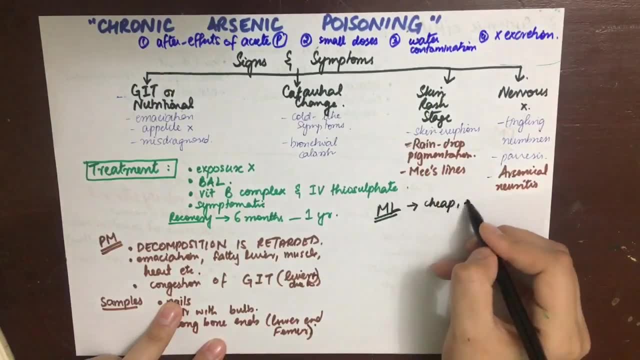 Samples of hair and nails should be taken. Hair should be complete with bulb and nails should be whole, Long bones and like femur can be used to detect the poison. Now the medical, legal aspects. The advantages of arsenic to use as a poison is that it is cheap, easily available, tasteless or doeless, and the symptoms are delayed. so the culprit has time to escape.